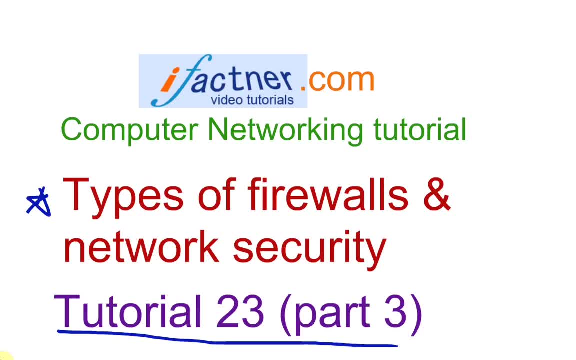 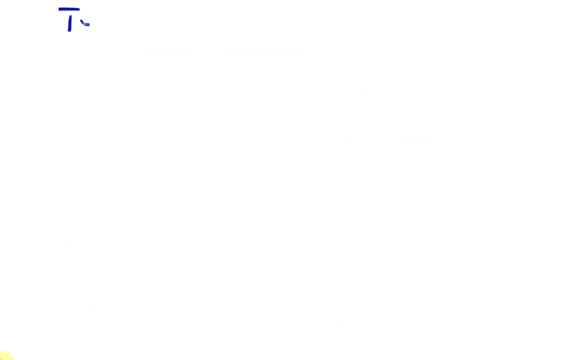 In the second part, we discussed about the generations of firewalls and in this part, we will be discussing about different types of firewalls that are available in the market. So, guys and girls, you would be happy to know that we have already discussed some types of the firewalls in the second tutorial, that is, the generations of the firewalls, and we 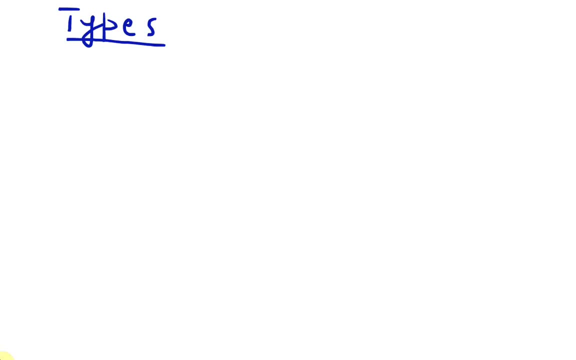 would be further discussing those types. So first type of the firewalls are called packet filters and we have already discussed that. there are two types of packet filters. Number one are the stateless packet filters that were introduced in 1980. And they only checked the authenticity of the packets. and the second type of the packet 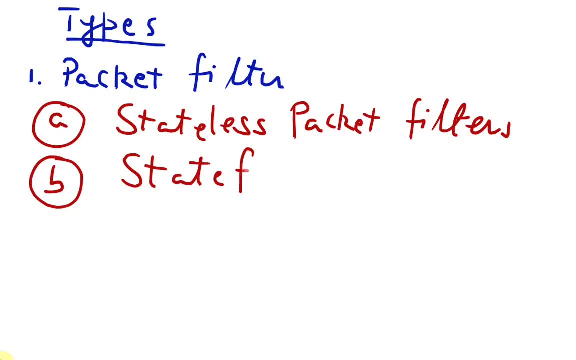 filters are the stateful packet filters and they check if the packet is a part of the existing communication or if it's the part of a new communication or if that packet is not a part of any communication And based on these three states, it can decide what to do based on the predefined rules. 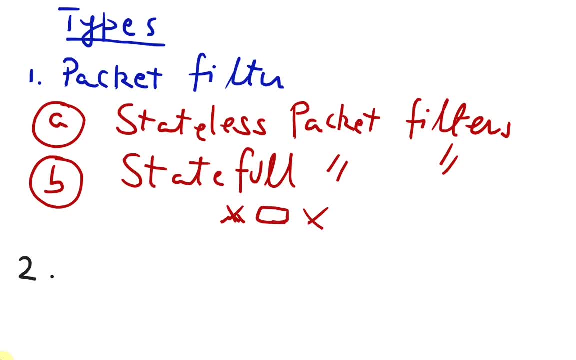 And the second type of the firewalls which we have already discussed in the generations of firewalls is called the application layer firewall. So application layer firewall mostly works in combination of packet filters, especially the stateful packet filters, and it works on the application layer of the firewalls. 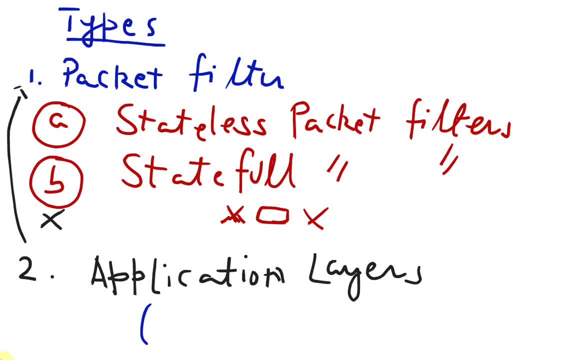 and it can basically check the authenticity of the packets, the connection status and the ports and the protocols of the packet. and if those ports and protocols are allowed, then application layers for filters would allow the packet to either enter into our system or the network or to go out to the internet. 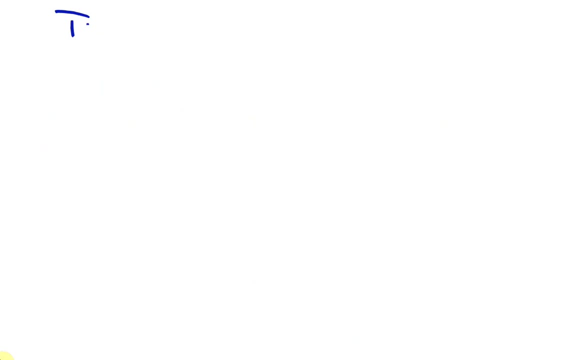 And the third type of the firewalls which we would be discussing today are called proxy servers or the proxy firewalls. And the fourth type which we would be discussing are called the NAT firewalls or Network Address Translation firewalls. Some people say that there is another kind of a firewall that is called the new generation. 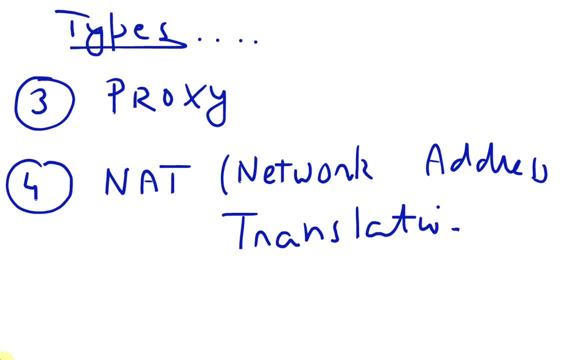 of the firewalls, But I would say that they are just the NAT firewalls. If you look at the top left here, these are the fourth type of firewalls, And the fourth type which we would be discussing are called the NAT firewalls or Network Address. 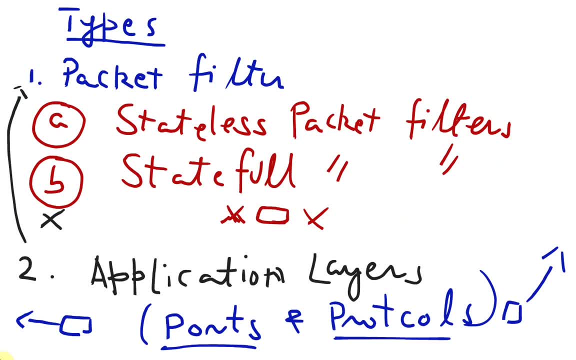 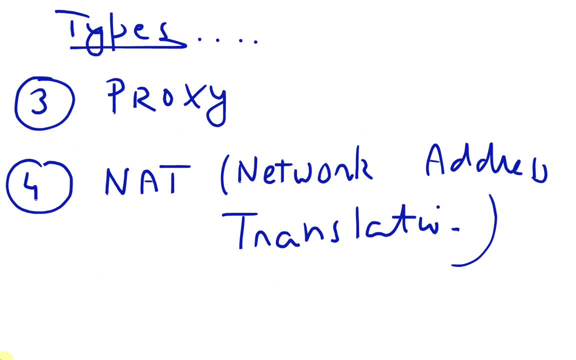 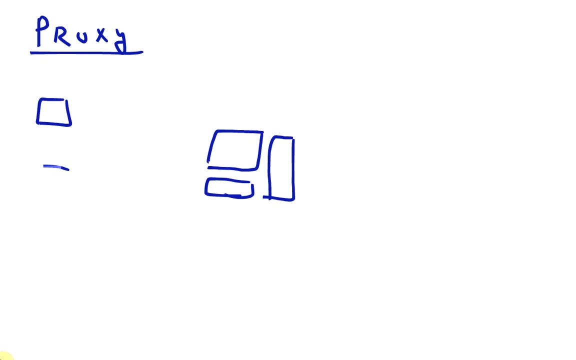 the newer version of the application layer firewalls, and they do the deep packet inspection. So now let's discuss about proxies. So first let me tell you what is a proxy server. A proxy server- you can think of a proxy server as a server which sits between your local. 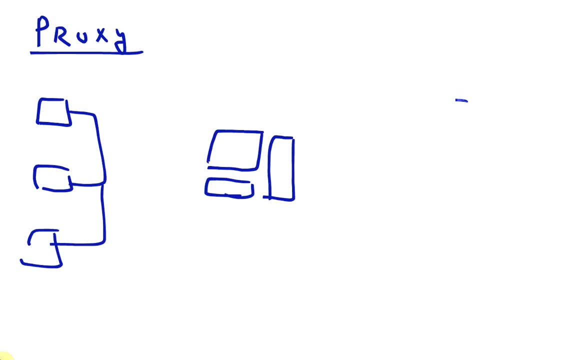 area network and the external WAN or network that are the internet, And all the communication is done via this proxy server. So you can think of it as a firewall, because in this proxy server we can allow the protocols that can be used. So you can think of it as a firewall, because in this proxy server we can allow the protocols that can be used. 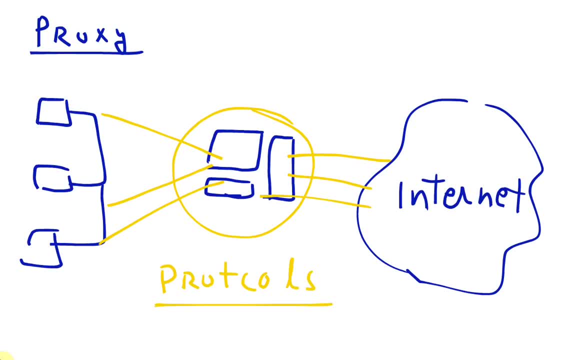 For communication, the ports which are open and which are closed. we can also define different set of rules. we can block the websites or different services of the internet used by security users. The advantage of a proxy server is that if you have got one internet connection, they 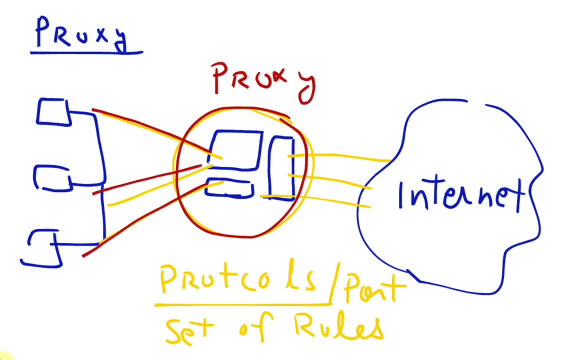 connection and we would like to share it with all the computers on our network. then we can use the proxy servers and the proxy server access and firewall, because it it is between our computers and the internet and it prevents the unauthorized packets or the unauthorized connection request not to go out or in. 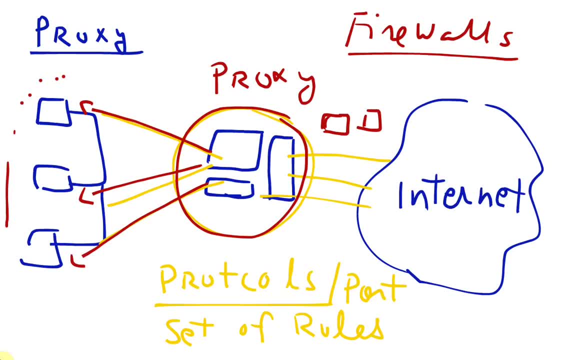 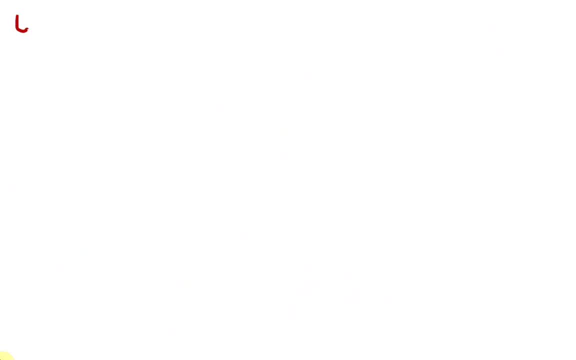 the system. so these are called the third type of the firewalls. there are the proxy server. the fourth type of the firewalls are called network address translation, or NAT, creation and integration of. so in an ideal case they would head to herbivore. in an ideal case. 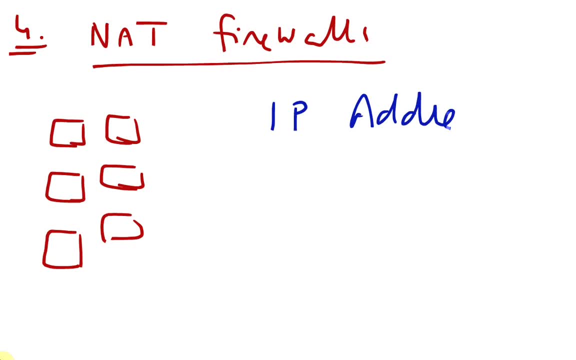 but we don't want to use the Call恨 by the public IP addresses and that would cost a lot of money. Therefore, a NAT system was developed based on which there are the private addresses and the private registerable and there are internal network addresses for each of the PCs in the 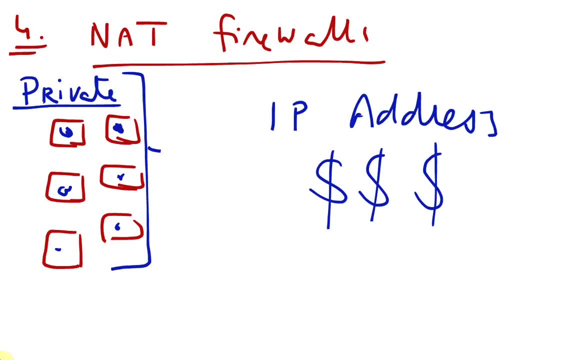 internal network and when the communication is turned to the external network through a router or a firewall, then that router or firewall or a computer system changes that private address into the public IP address and sends the packets to the internet. So in this case the internal network, the private addresses of the network, are secured. 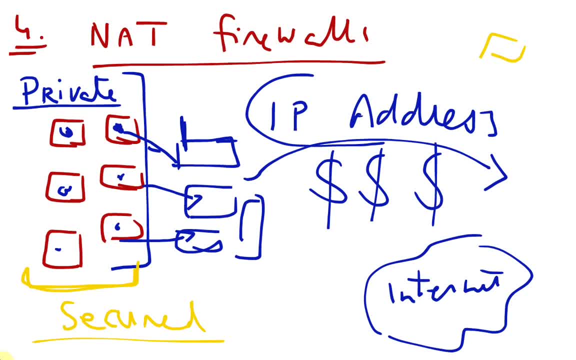 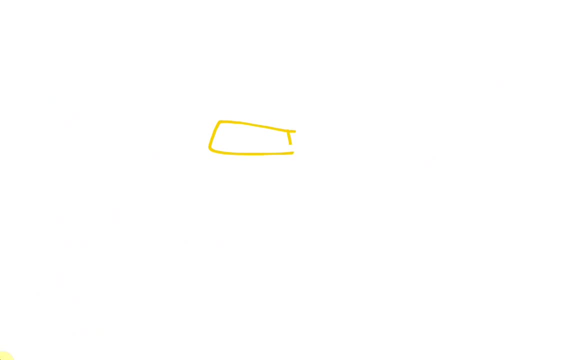 and the outside person or the outside computer may not know the internal IP address or the address of, for example, this PC. So the firewall acts as a bridge. So the firewall acts as a bridge. It screens the private IP addresses to be seen from the external users and it changes. 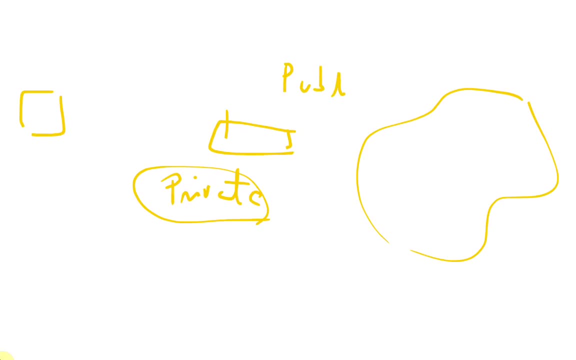 those private IP addresses into the public IP address. when those IP addresses passes through it and therefore those PCs which are on our internal network, they are secured. And nowadays the IP addresses are secured And they call a new type of a firewall, but it's an older type and it is called New Generations.